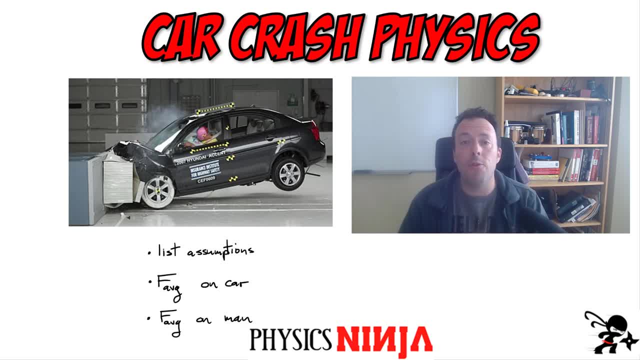 on the car? What is the force on the man? Now we're going to have to make a couple of assumptions when we try to simplify this problem, because you can imagine how complicated it is. with the car kind of coming into contact with this concrete block, There's a lot of different materials at play with. 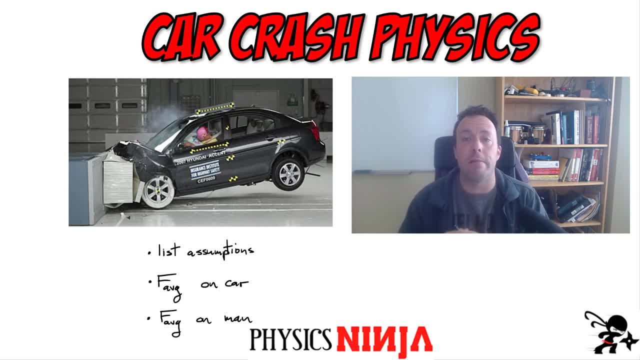 a lot of different properties. but how can we analyze it? just using basic physics, making realistic assumptions. Okay, so we're first going to do some of the math to set up an equation to calculate the average force. Then we're going to plug in some numbers to get an order of magnitude. 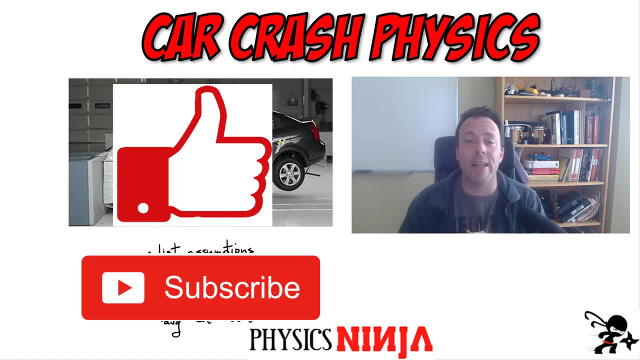 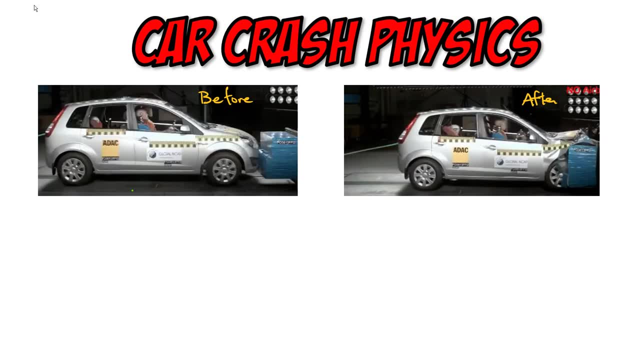 of the car. If you like it, give it a thumbs up. Consider subscribing to my channel. Okay, let's get started. All right, so let's have a look at just some of our statements here. So we have before and after. So before we have this car that's traveling to the right here at some velocity. Okay, so we're. 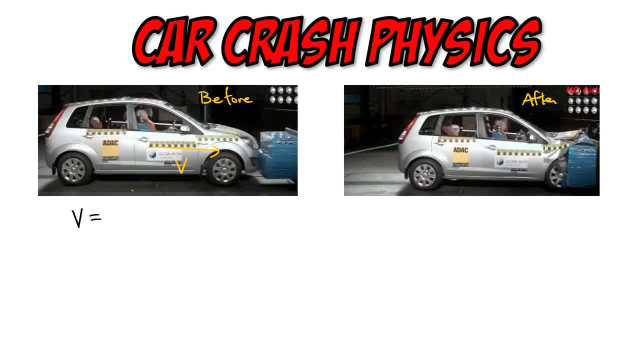 going to assume now that the velocity is going to be quite high. Let's say it's 60 miles per hour. Okay, so first thing I want to do is maybe convert that into meters per second so I can calculate the force in Newtons at the end of the day. So I want to get rid of miles, Maybe get. 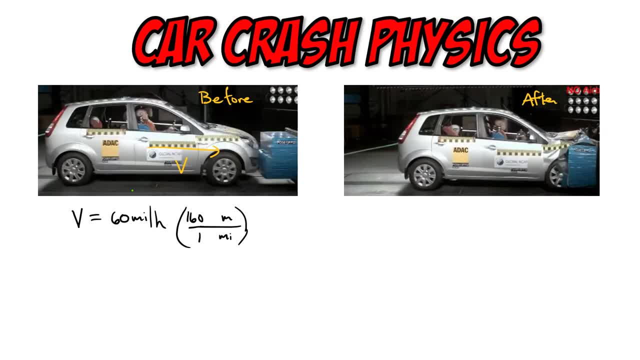 meters over here. I know in one mile there is like 1,609 meters. And then I can also get rid of hours And I want to get seconds at the end. I know in one hour there's 3,600 seconds. So if I 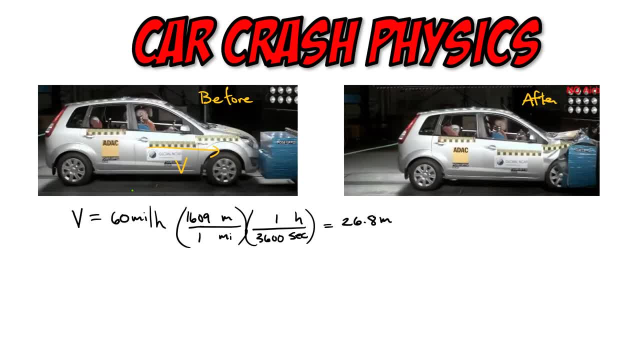 do this conversion, I get 26.8 meters per second as my speed. Okay, so that's my initial speed. My final is 26.8 meters per second. So that's my initial speed. So that's my initial speed. 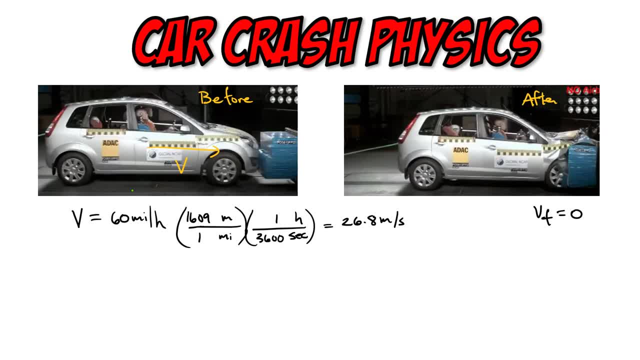 The final here has to be zero because you come to a stop. So this is going to be my initial velocity. Now I'm going to look at two things. I'm going to look at the man. Okay, the man here is going to. 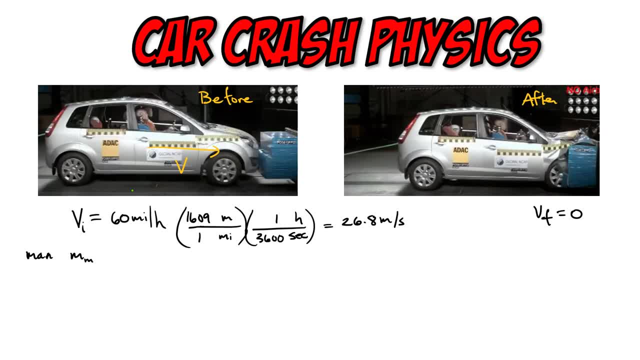 have a mass, The mass of the man. we're going to assume here it's 80 kilograms. I'm going to look for what is the force acting on the man? And then there's also the car. Okay, so the car has a much. 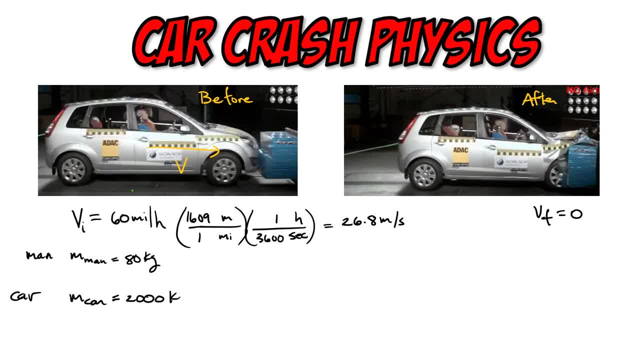 bigger mass For this problem. I'm going to assume that the car has a much bigger mass, So I'm going to assume it's 2,000 kilograms. Now, a couple other things we have to look at now is look at the. 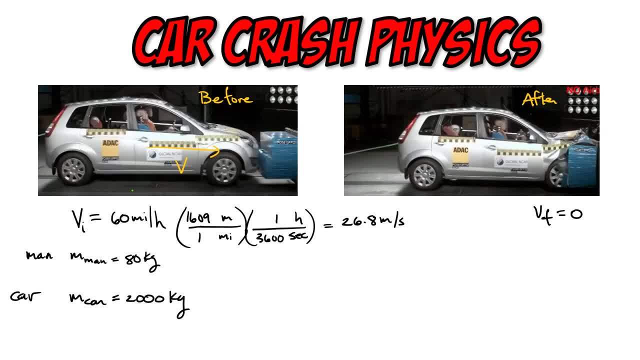 stopping distance. right, This car here compresses a little bit. right, You can see, it compresses probably from the start of the car all the way to this distance here. This is going to be my stopping distance. So my stopping distance, let me just write this down: Stopping distance. 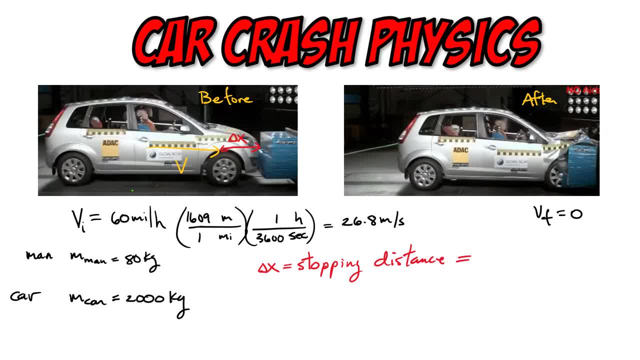 It takes a certain amount of distance. right, This force is being applied over a certain distance And for this problem, I'm going to assume, just based on this diagram here, it's approximately 0.5 meters. Could be a little bit smaller than that, could be a little bit bigger, but let's. 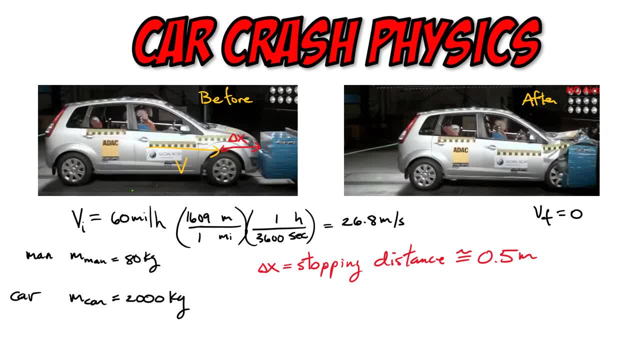 just make this assumption. This seems to be a reasonable number. Okay, the other thing that we're going to have to assume in this problem here is we're looking really at an average force. Okay, actually, if you would plot what the force. 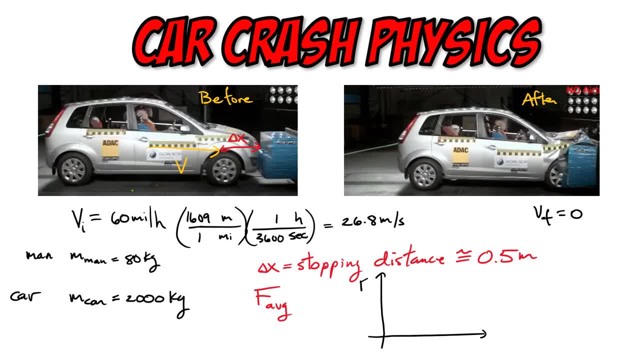 looks like as a function of time for this car accident. you know, it might start off really small, It might end up being something pretty big and then go back down close to zero. This is probably more realistic, Okay, what we are doing here by just looking at an average force. 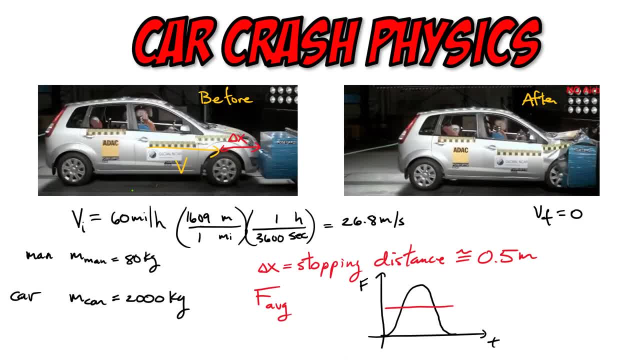 we're going to assume that the force here is some average value and it's uniform throughout the whole time here where this compression is happening. Okay, so this is an assumption That we make. Okay, so we assume that this average force here is going to be a constant value. 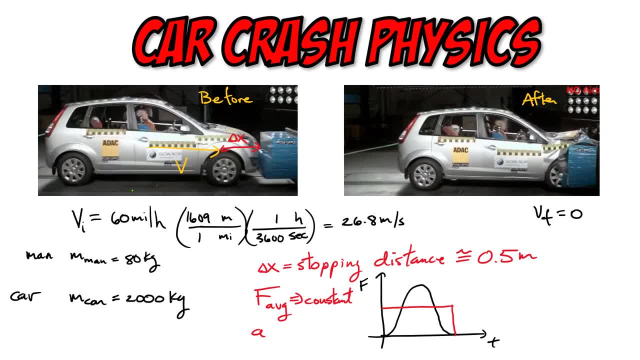 Okay, that also means that the acceleration of the car is also a constant. If the force is constant, the acceleration must also be constant. Okay, All right, let's go down on the other page and figure out what equation I need now in order to calculate what this average force is. 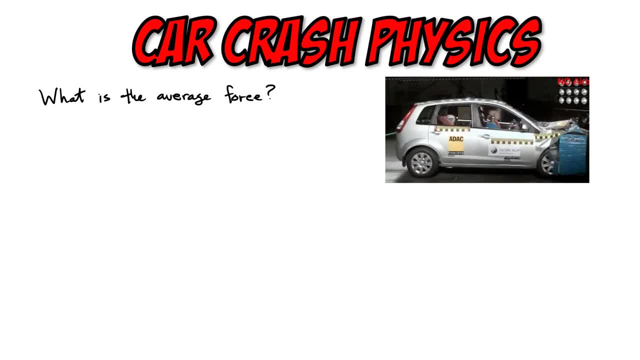 All right. so what is the average force? And again I'm going to have this displacement here of Delta X, which I assume is about a half a meter. How do we calculate average force? Well, again, there's going to be a force acting on this car and the force is a stopping force, So it has 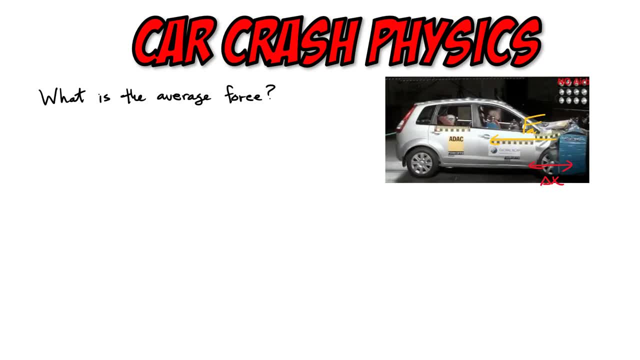 to be to the left right. That is going to be my average force. How would we calculate what this average force is? Well, one way you could say is that this average force is going to be equal to the mass times, the acceleration or the deceleration of this car. right, This car is going to slow down. 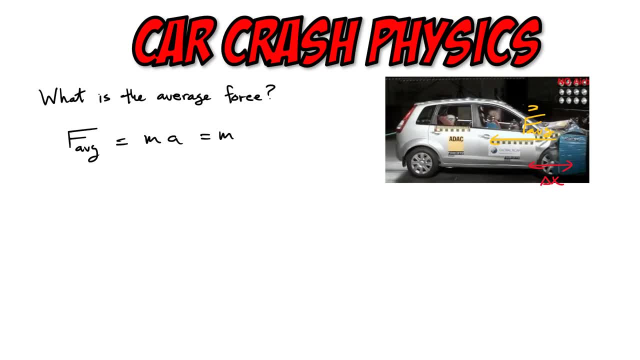 So let's take this a little bit further. What is my definition of acceleration? It's the change of velocity over the change in time. All right, I can bring this down a little bit more. Delta V is always a final value minus an initial divided by Delta T. How much time does it take to stop that? 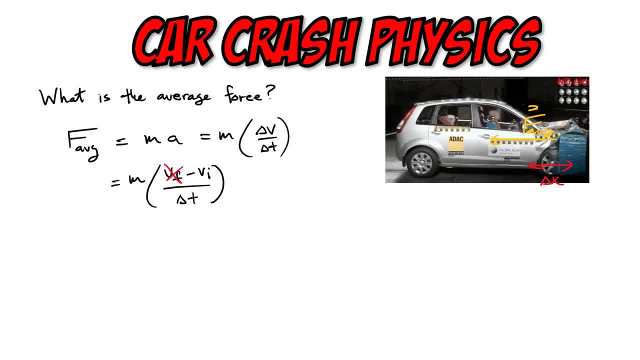 car. All right, so V final is zero. That's a simplification we can make. So let's just look at this equation. I'll bring that negative sign to the front: V I divided by Delta T. Okay, so we're getting there. So it depends on the mass, depends on that. 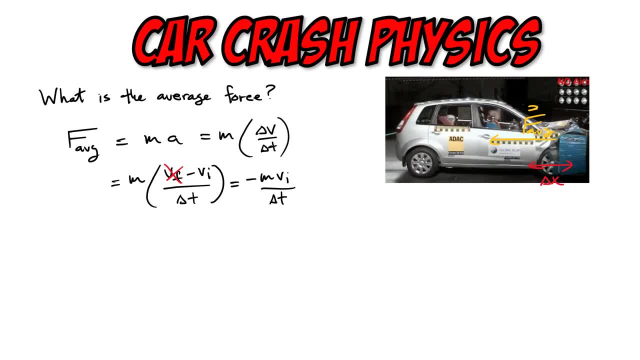 initial speed, but also depends on this time. Actually, what I want to do now is I want to eliminate this time and get it in terms of this Delta X. Okay, so how can I do that? Well, so now you have to think about the kinematics of what is going on. Okay, Delta X is going to be equal to. 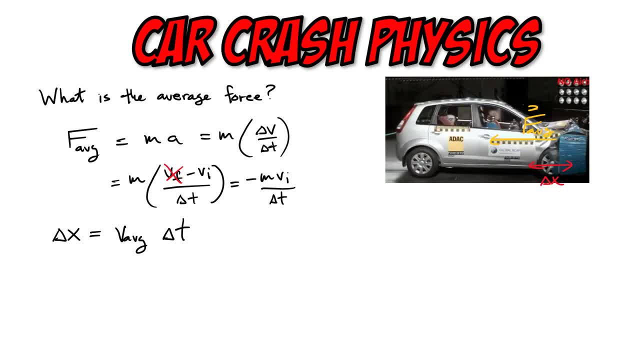 an average velocity multiplied by the speed of the car. So I'm going to do that. I'm going to multiply by the amount of time. Okay, and this average velocity is just one half V initial plus V final, and multiplied by Delta T. Okay, now again, the V final is zero. So that's an easy. 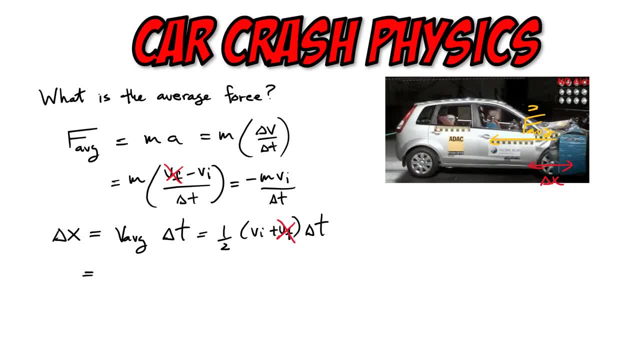 simplification we can make So that Delta X distance is one half V initial, multiplied by Delta T. Again, all of this is assuming that we have a constant acceleration right, That the velocity is changing uniformly. Okay, so let's go ahead now and substitute this Delta T inside my average force equation, So I get. 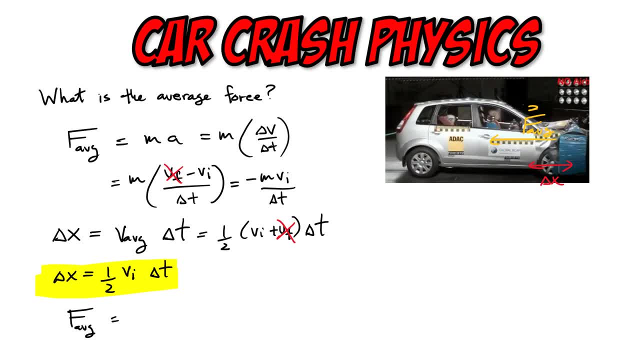 finally, that my average force is equal to minus MVI and, divided by now, Delta T, So Delta T. you have to just do a little bit of algebra. Bring the two over here, Bring the VI at the bottom, So you get two Delta X. And then there's another VI. I get divided by VI. I just bring that one to the top. 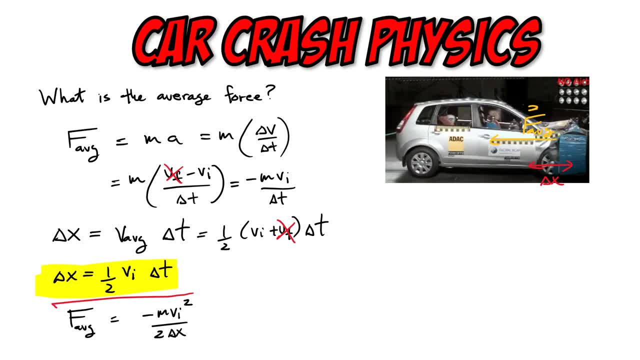 All right, this is my expression here for the average force acting on any object of mass M that started at an initial velocity and that had a final velocity equal to zero. If you wanted to, you can also use a work energy theorem in order to get this result. Okay, I'll show you how to do that real quick And the reason you can use. 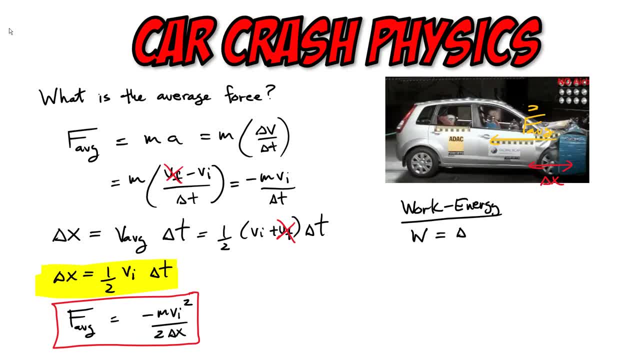 this again: the work done by any force is equal to the change of kinetic energy of an object. Well, this is a final value minus an initial value. The final kinetic energy has to be zero because I come to a stop. My initial kinetic energy is one half MVI squared. 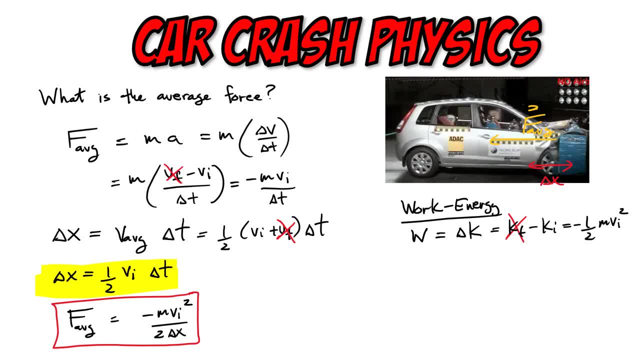 You can see some of the terms are starting to look quite similar. Now how do I calculate the force or the work, rather, The work, you can simply write it as a force. In this case it is a constant force multiplied by a displacement. 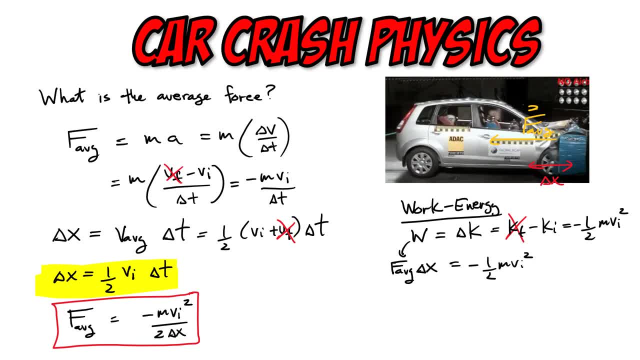 All right. so that becomes minus one half MVI squared: Okay, initial squared. so at the end you get the average force minus m VI squared over 2 Delta X: okay, it doesn't matter which method you use. if we make the same assumptions of a constant force, we're able to get to our expression. so now, 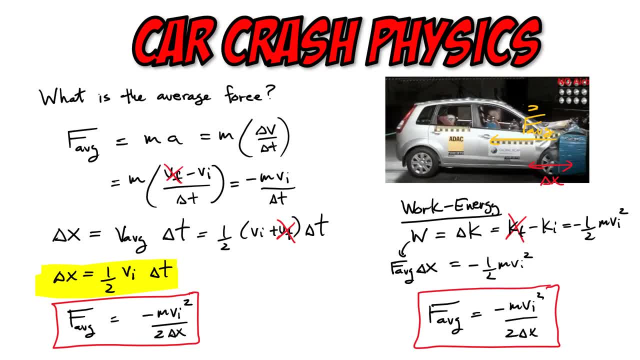 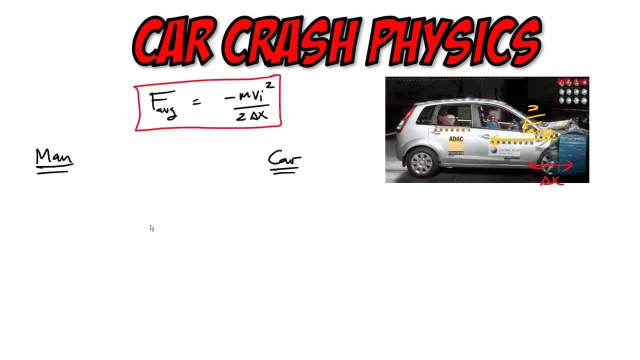 what we want to do is go back and substitute our masses and our initial velocities and have a look at what these forces equal to for this problem. all right, let's plug in some numbers over here. so for the man we set, the mass is going to be approximately 80 kilograms. for the car, say mm for the man, MC. for. 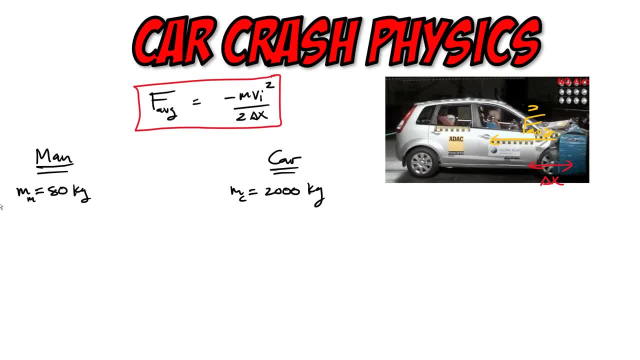 the car 2,000 kilograms. you can see that the mass is an enumerator, so it's a much larger force on the car. clearly, that initial velocity is going to be the same for both: 60 miles an hour, which we converted, so we have 20 miles an hour and we have 15 miles an hour, so it's almost like 20. 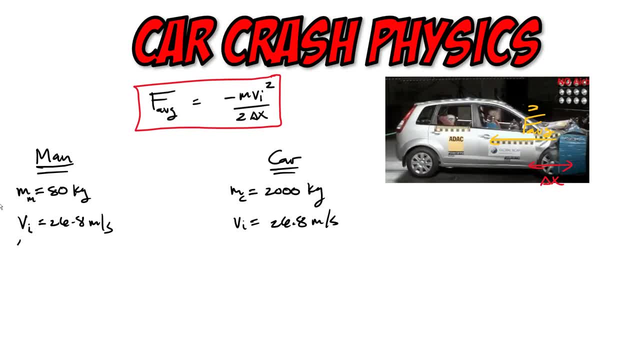 26.8 meters per second. what else? and the stopping distance is going to be? let's just set it equal to the same delta x equals 0.5 meters. okay, so now we just substitute the numbers. uh, if you're worried about that negative sign, negative sign, just tells me the direction. right, the direction is clearly. 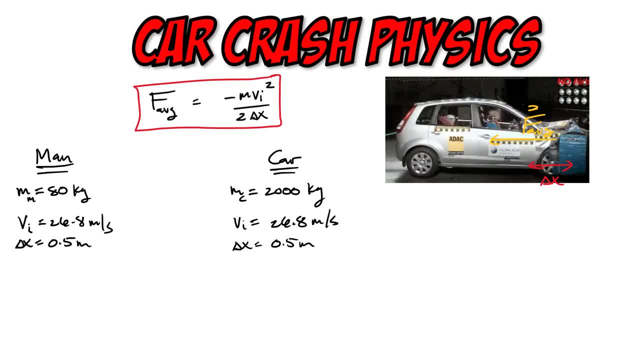 opposite of the displacement. the displacement is moving forward, uh, by half a meter. the force is acting in the opposite direction, which is why you have that negative sign. but if you're just worried about the magnitude, uh, let's just forget about that negative sign for now, and let's just substitute. 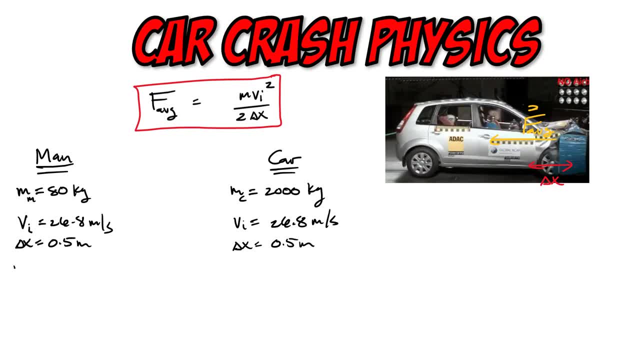 our numbers see what the average force is. all right. so the average force on the man, all right. so i would do, uh, 80, 26.8 squared, and then two times 0.5. all right, you calculate that average force on the man and i get approximately 57 000, say four. 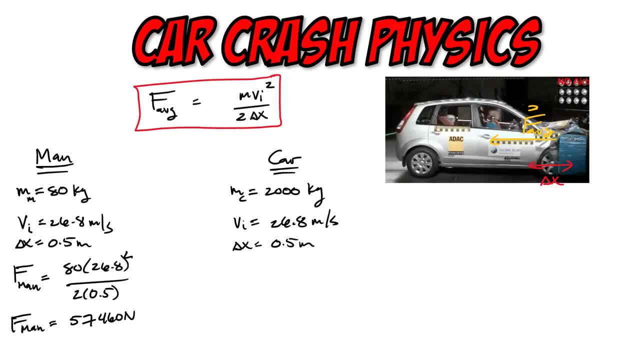 six, six the newtons, all right, pretty big. how about on the car? on the car again, just substituting, just really the mass is the only difference here is 2000. when i substitute the numbers i get a giant number: hundred. wait, one, four, three, six, four, eight, zero newtons, wow, uh, let's calculate that in. 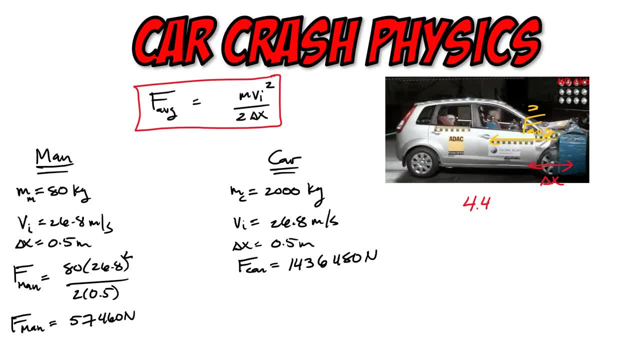 different units, right, sometimes, force you can calculate in pounds, right, uh, the conversion factor is four point uh. four five newtons is equivalent to one pound of force. so all you have to do to convert the pounds is just divide by 4.45. if i do that for the man, uh, calculate that in pounds, i get approximately twelve thousand. 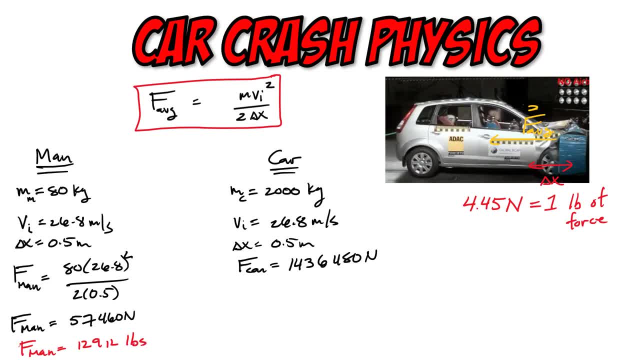 nine hundred and twelve uh pounds of force and for the car i'm getting approximately three hundred and twenty two thousand, say eight hundred, approximately pounds of force. okay, so that's kind of how you would calculate that. you can also calculate what the average acceleration is once you know the force. you just divide by the mass. okay, my average. 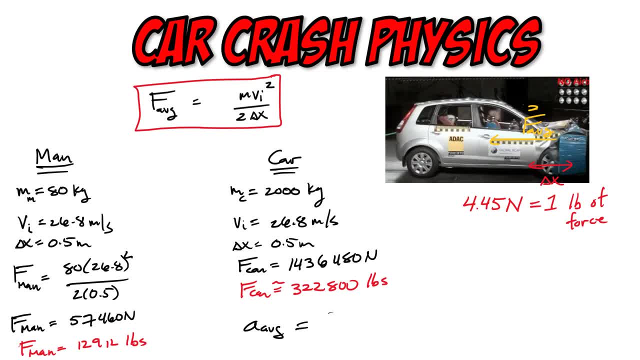 acceleration for both objects. um is just the force, the average force divided by the mass. so either you take the man or the car value, you just have to divide it by its respective mass and you're going to get the same value for both of them. i get for this particular case like this one- here is the man. 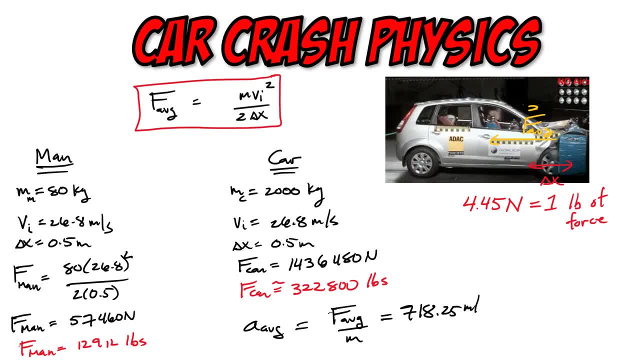 like 718, say 0.25 meters per second. uh, if you divide that by g you can calculate that in g's, and little g is 9.8. so if i do that, i get approximately 73.3 g's of acceleration okay, which is uh kind of. 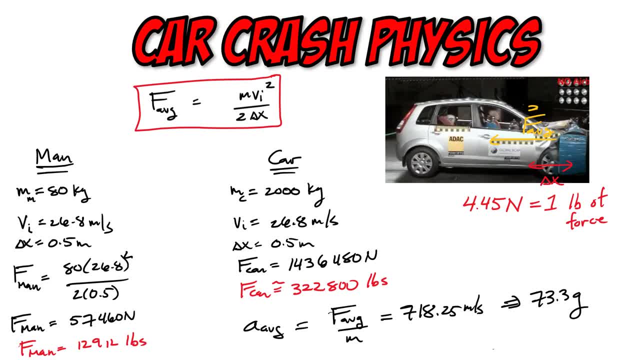 a very, very large number right compared to just the acceleration due to gravity. right, we have 73 times the acceleration due to gravity just for stopping this object. all right, let's kind of have a look now at some charts and see, uh, just have a look at this equation in more detail, okay, what? 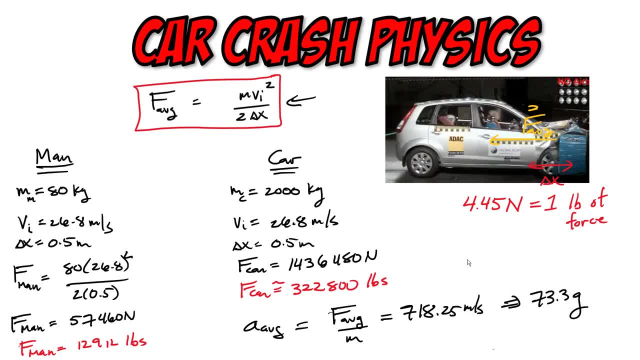 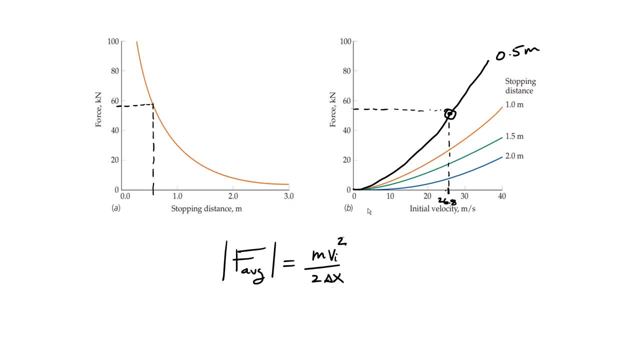 happens if i increase the stopping distance? what happens if i'm traveling faster or slower? all right, let's have a look at this equation in more detail. all right, last thing i want to do is just kind of uh, just plot um what the average force looks like in terms of some of these parameters. 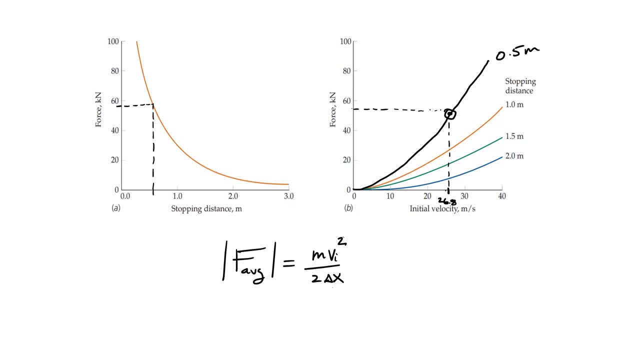 okay, the first thing we can do is play around with the stopping distance. okay, you see that the stopping distance appears in the denominator right here on the left hand side of the graph and the right side of the graph. right here on the left hand side of the graph, which is the force that the 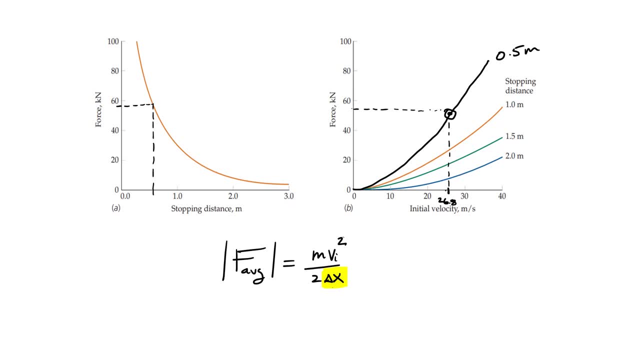 force larger. so which means that if i make it bigger, i'm gonna make the force smaller. okay, so the first chart i show here on the left hand side here is this force in thousands of newtons and kilonewtons versus this stopping distance. now, the case that i considered here was: 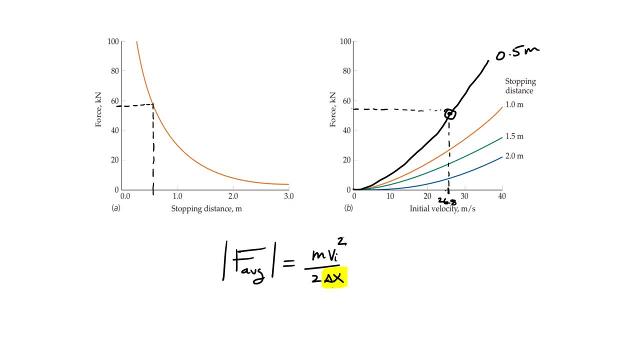 um, the stopping distance of half a meter, and then i got a force of Okay. so this is force on the man. Okay, you can see now, as I make that stopping distance bigger, if I go to one meter I get something like 30,000.. 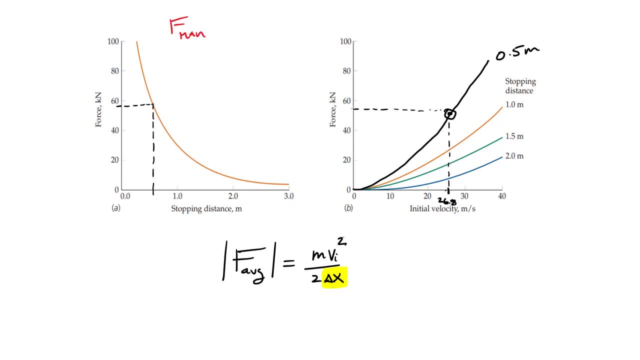 If I go to two meters, I get something around 10,000 from the chart. Okay, so increasing that stopping distance plays a big role in reducing that average force. All right, the other thing you could look at now is for a given stopping distance, right? 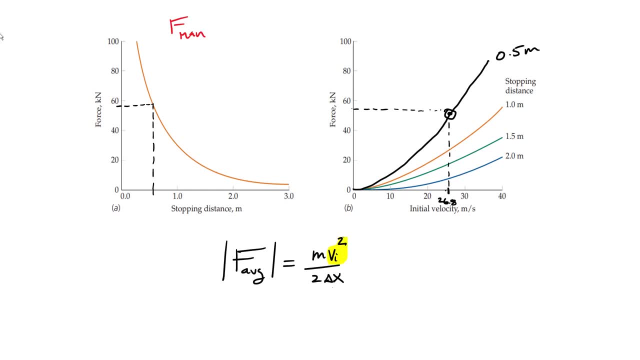 What does it look like in terms of this initial velocity? Right? you see, the initial velocity term shows up here as a squared term, So that actually is a big dependence on it, right? If you plot any of these curves of average force- again, force on the man. 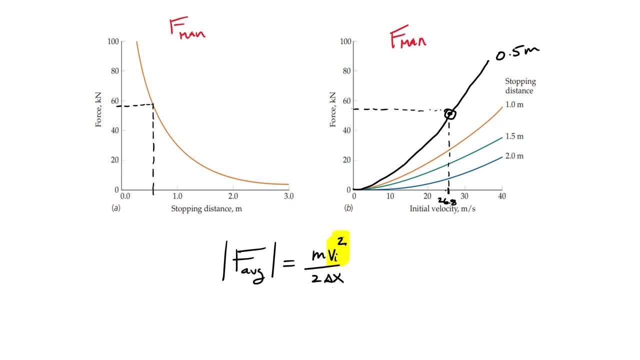 Let me just be explicit here: Force on the man versus this initial velocity. they're always going to have this quadratic dependence here, right? They're not straight lines here, right? These are kind of growing pretty fast, these curves The different colors here represent.